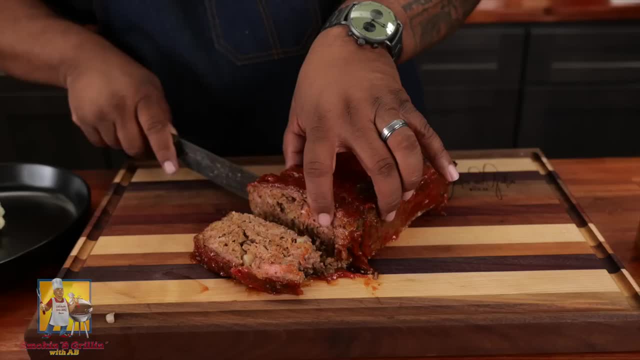 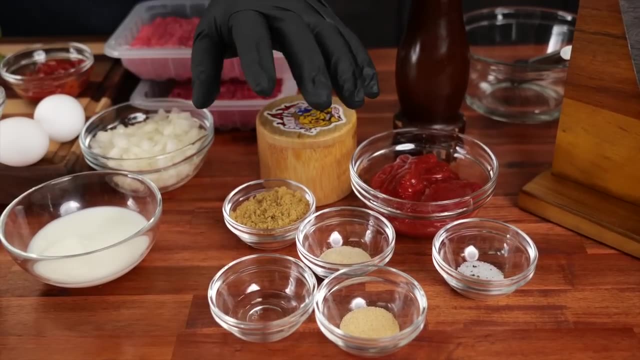 Hey, check out this meatloaf right here. Listen, it's budget friendly, it's easy, it's moist, and check it out. that sauce that we're going to put on the top is killer. Let's get it. First thing you want to do is you want to measure out all your ingredients. for those of you guys who are going, 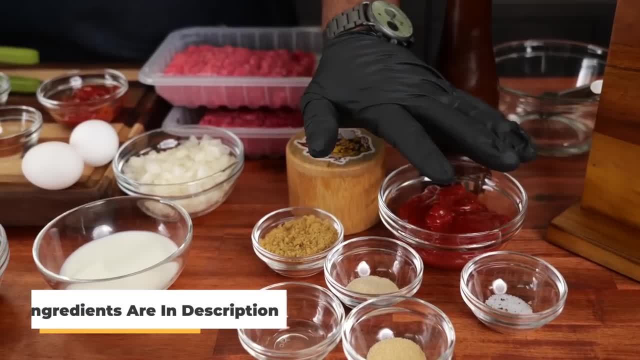 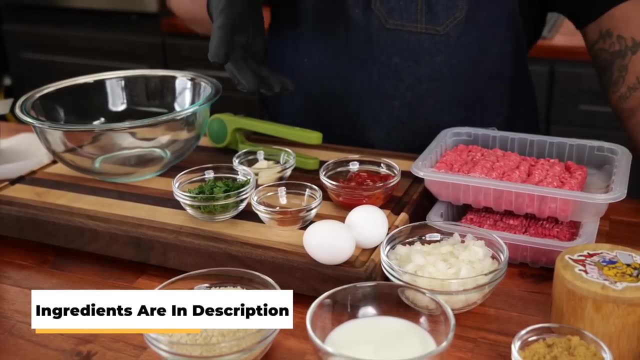 to be doing the measurements right. So, look, I got the glaze and everything over here on this side and then, if you look over here, I got, you know, the ingredients over here. This is everything that's going to go inside the you know with the meat to. you know, make the meatloaf right, Hey, and 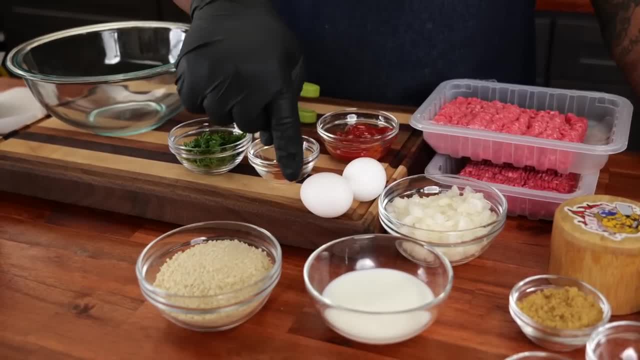 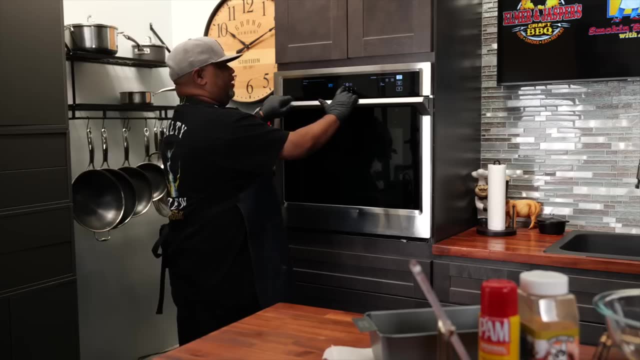 as always, the full ingredient list with the measurements will be down in the description box below. Let's get it. Okay, look. so the first thing I'm going to do is I'm going to preheat my oven. right, I'm going to preheat this to 375 degrees. This, right here, is what I use for the. 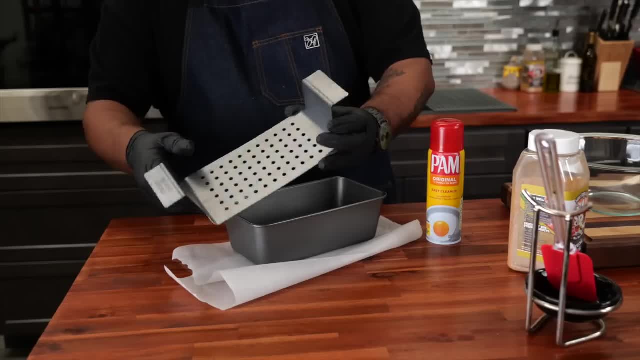 meatloaf, right. Look, I want you to pay attention to that. It's got the holes in it. So listen, a lot of people tell you you want to use like 90-10, you know, a leaner meat, right, But this way you can use. 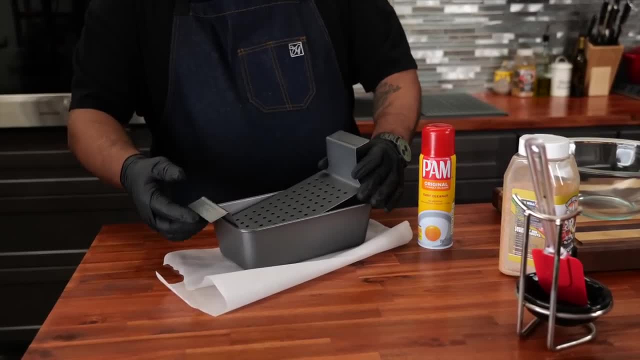 I've even used 73-27, but I like to use 80-20, right? You set it in here, you form it. then when you take it out, what does it do? It drains. Now, for those of you who don't know what it does, it drains. 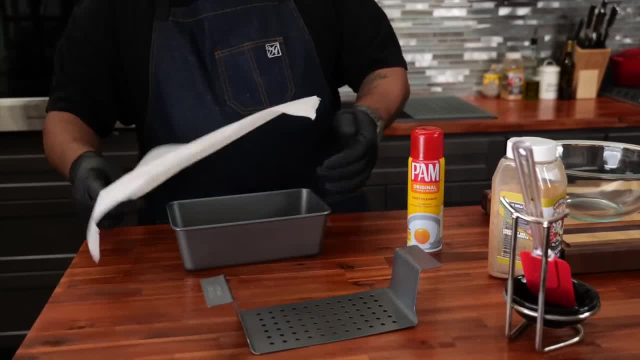 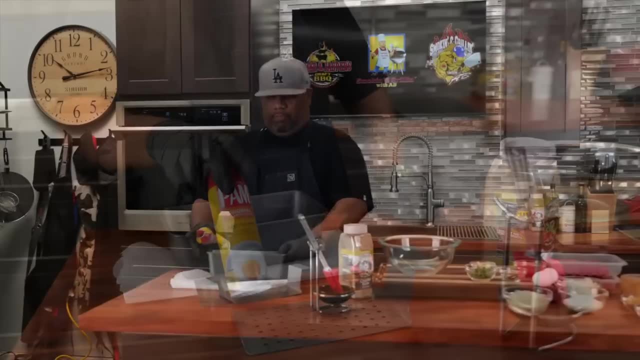 You guys don't have, you know, this apparatus to go inside of there. you can always get yourself some parchment paper and do it, or you can do it old school like me, like I used to do it, and we just come with the pan. Okay, so, since I got everything set up, remember the parchment paper for those you 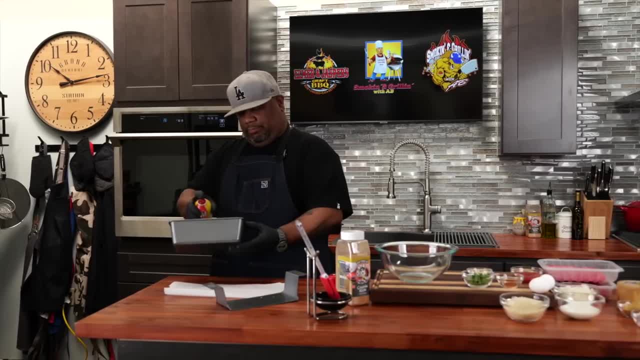 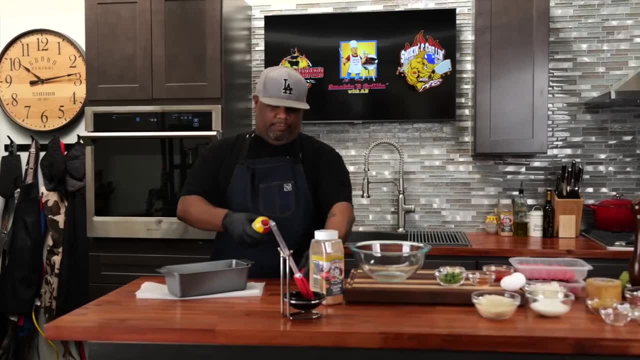 guys that don't have. you know this right here. but I'm gonna go ahead and just spray it just to make sure nothing sticks on the side, right. And then of course I'm gonna take this spray just the bottom of it and we just let this sit up and then we work. So when I tell you it's a dump and go. 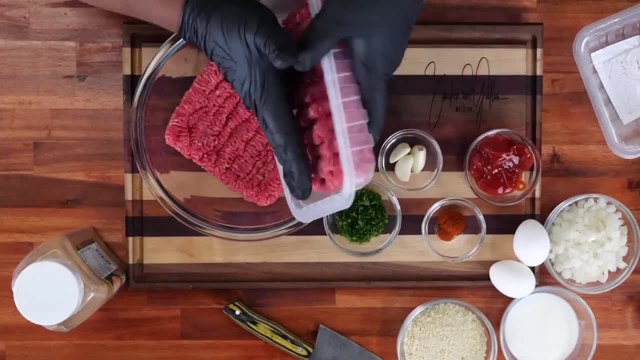 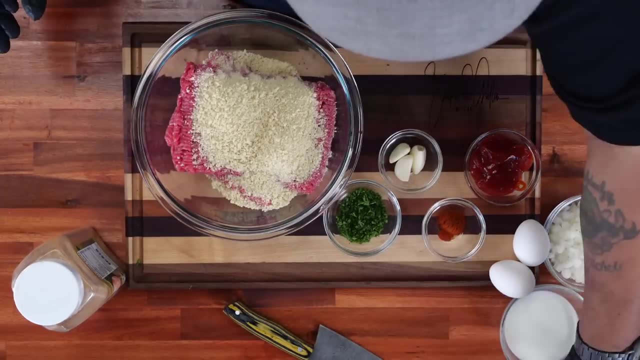 it's a dump and go right, So I'll go ahead and spray it. Look how fresh this ground beef is. This right here is 80-20. just you want to put everything in here. Now that I'm looking at my bowl size, probably wish I'd have got a bigger bowl. you. 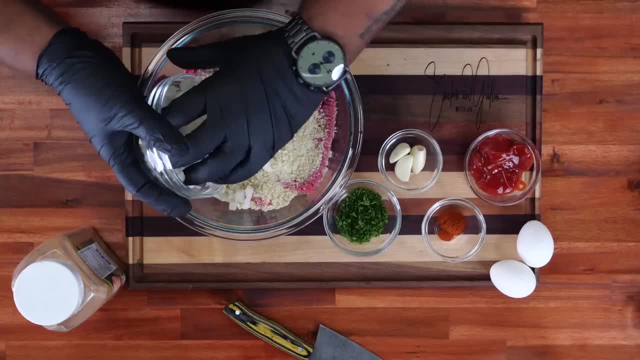 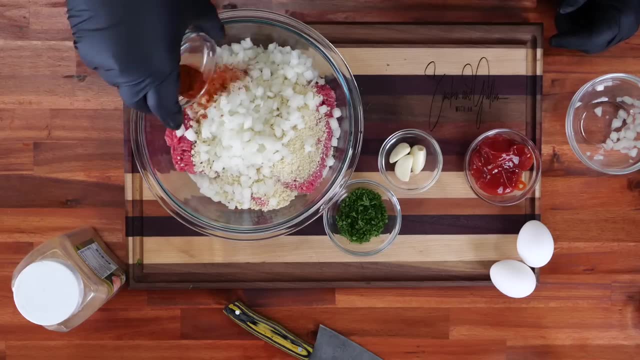 know, but we'll work with it. Add some of these onions. I like a lot of onion in there in mine. I'm gonna hold something back right, This, right here. just sprinkle our seasoning on the top. Now you guys use whatever seasoning you like, but right now I'm gonna go ahead and just get you. 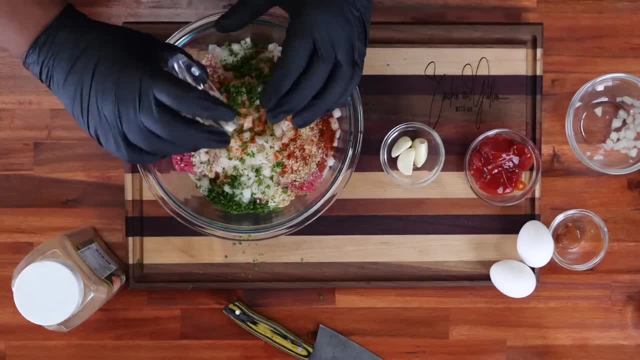 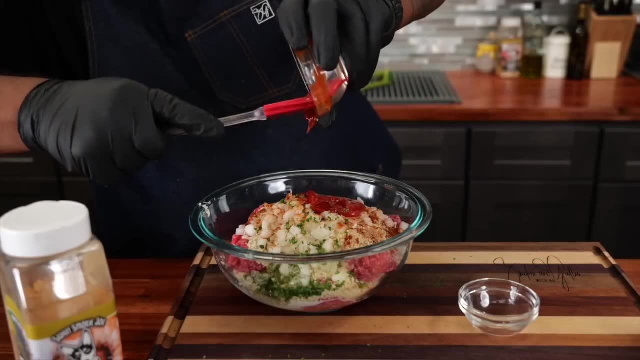 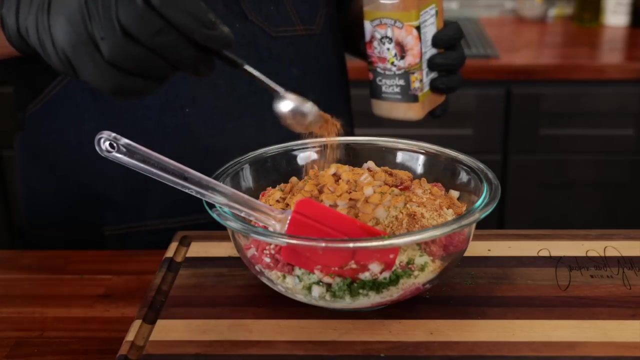 in the ballpark. You know what I mean. For me, I like to use everything Creole. So look, now I'm putting in the Creole kick. right, I put in about a tablespoon. Listen, it's the perfect blend to give it that kick. Now, if you guys want to, this is where you probably put in two table. 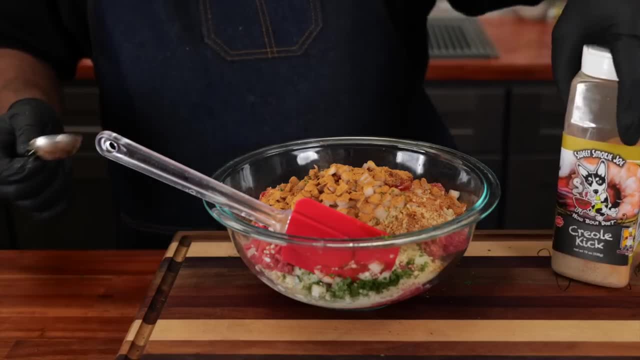 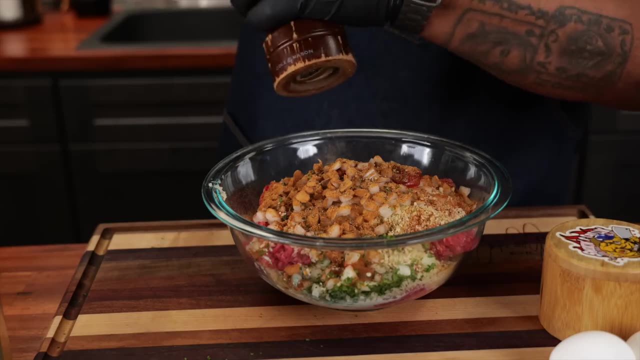 two teaspoons- listen to this- of Italian seasoning, That's. if you want to do that. Now we come with our pepper. Now I'm gonna hit it with pepper twice. You know what I mean, because this is only going to go so far. You know what I mean. Then, after I get it mixed- halfway get it mixed- I'm gonna add some more. 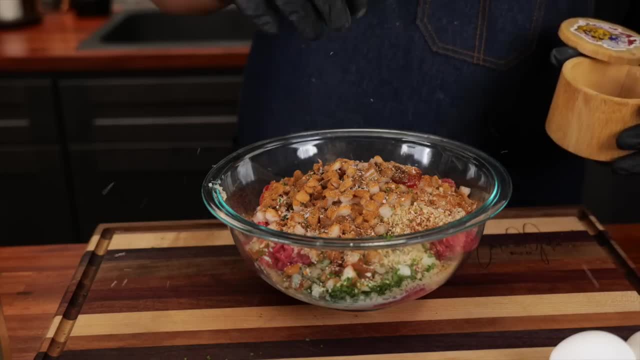 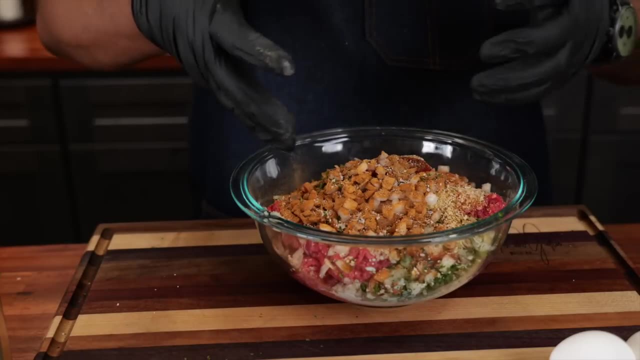 for the salt, I'm gonna do the same. I'm just gonna give it one generous pinch and leave it like that, and then we'll come back to it right? So now we're gonna get in there with our hand, and now what we're gonna do is we don't want to like just beat the meat up right, Like roll it all tight. 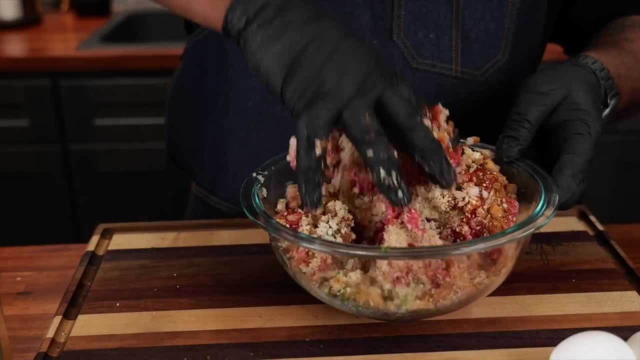 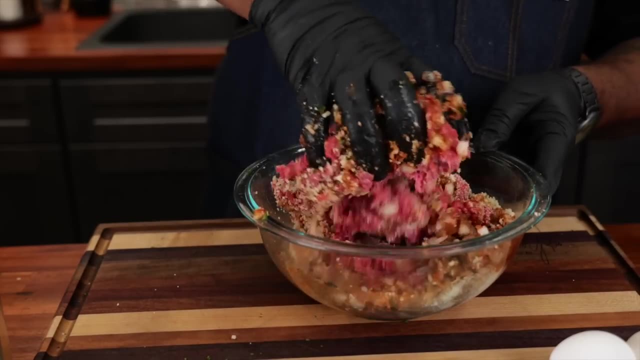 so we kind of like just gonna crumble it, you know, just like this, just to get it broke up right. Once I get it broken, then I'm gonna add these eggs. We just want to get it halfway and I like to make a little indentation like this. I don't know, can you guys see that I like to start like that, right. 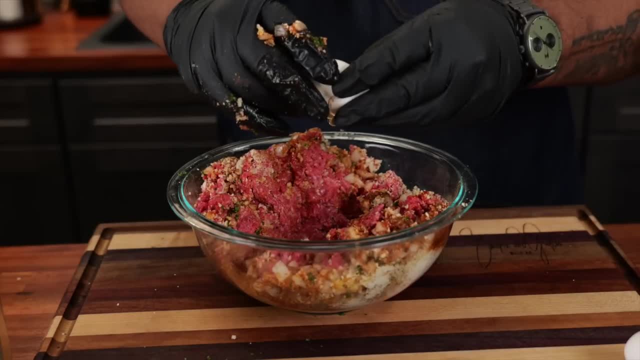 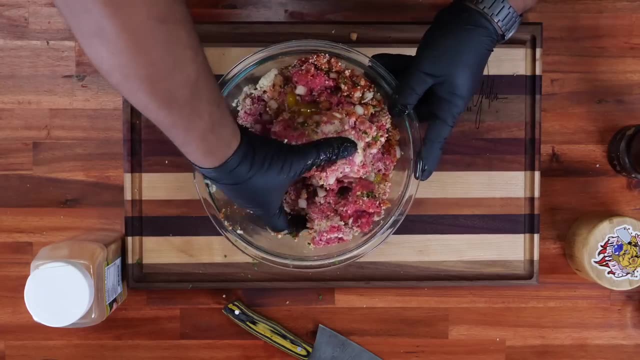 So now let me go ahead, open up an egg, Drop it in just like that, Check it out. We're just gonna fold it over, Make sure we break that yolk, and then we're gonna get it to start working down and some of the other meat. Now for me I just kind of like just fold it over and just work with it. 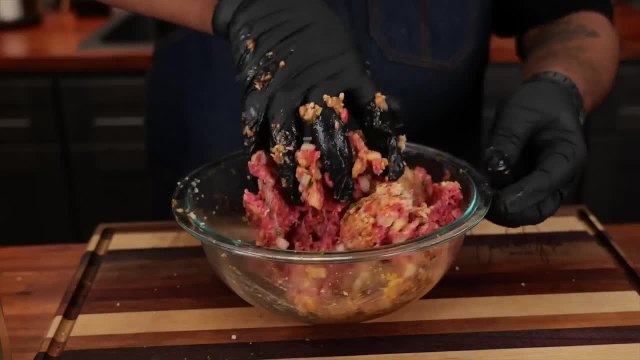 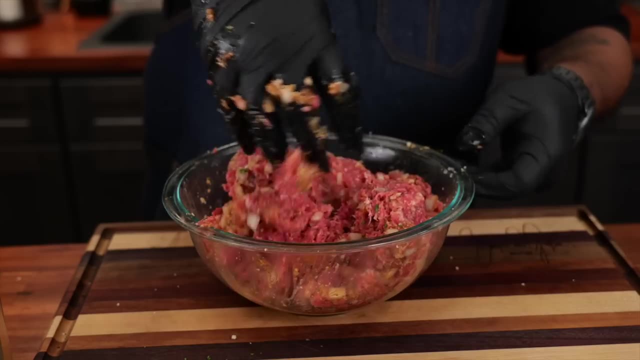 generously. Now let me clean these gloves off. You know what I mean. I want to go ahead and add a little bit more salt, Just one more pinch, and just a little bit more of the- uh, of the black pepper, and then we're gonna go ahead. 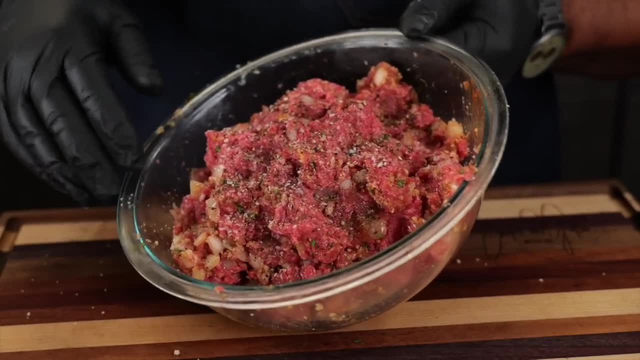 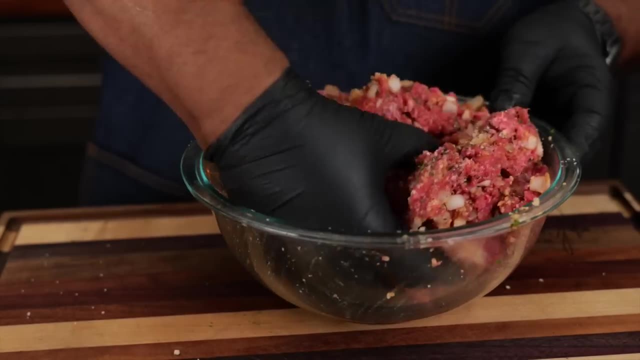 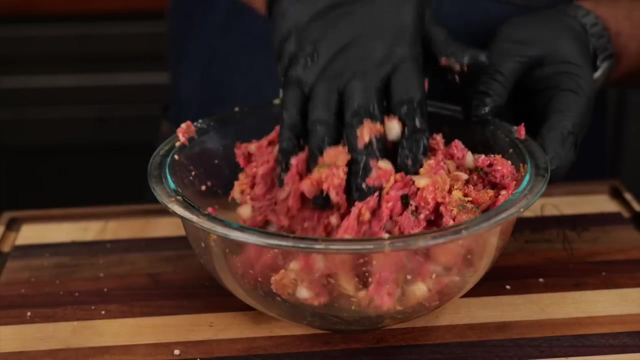 and form it. So look, as you can see. you can see the kosher salt on the top, You can see the black pepper. Now I'm just gonna give it, you know, a few folds over and this is it right here. You just don't want to overwork, you know your, uh, your ground beef. You want it to be as loose as possible, but you 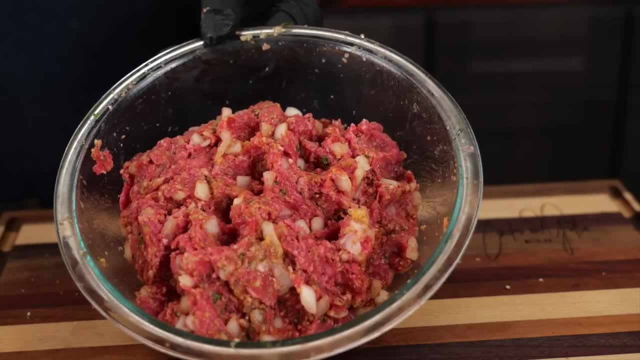 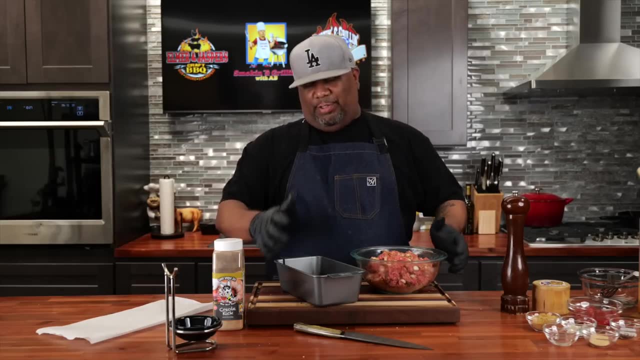 still want it to be thoroughly mixed. Look at that right there. That's what you want to get, Okay, so I brought my pan into this right now. You know, this is my meatloaf pan. I got to tell you this. You don't have to have one of these. You know you can get yourself a regular uh bacon pan, You know. 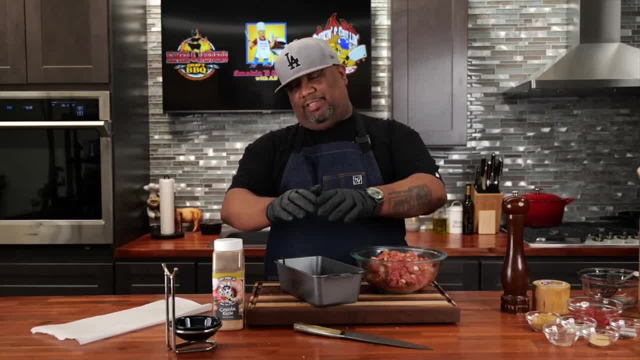 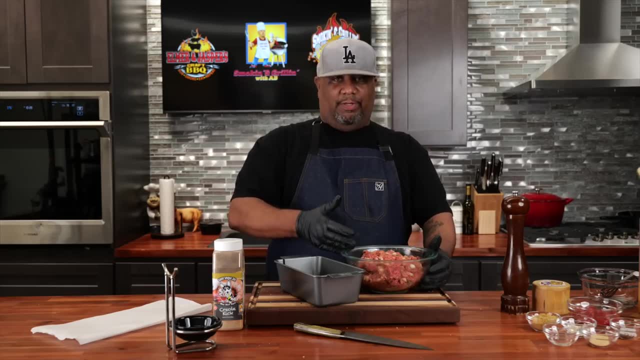 what I mean. You can spray the bottom of it, You can put this meat on top of that and just form it with your hands and do it that way. Now I'm gonna give you guys another little tip. Look, there's some things that you can do right now that you know like: level this up. I could have put cheese in. 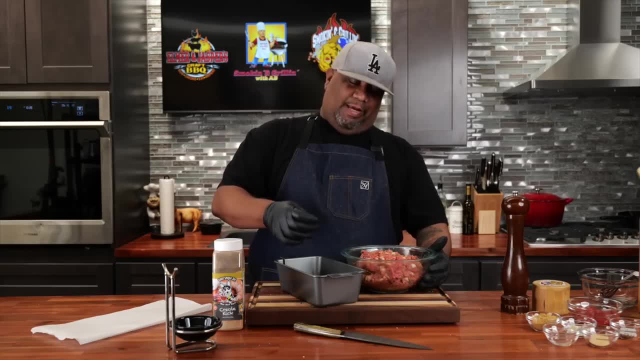 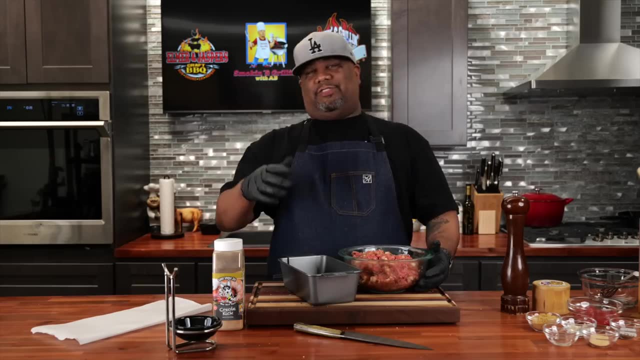 there. I could have sprinkled cheese, Made it like that, We could have put a little some A1 sauce and then, if you guys been watching some of my other videos, you know I use uh W sauce. Hey, and the W sauce. go ahead and answer the comment. You know, ask the question down in the comment section. 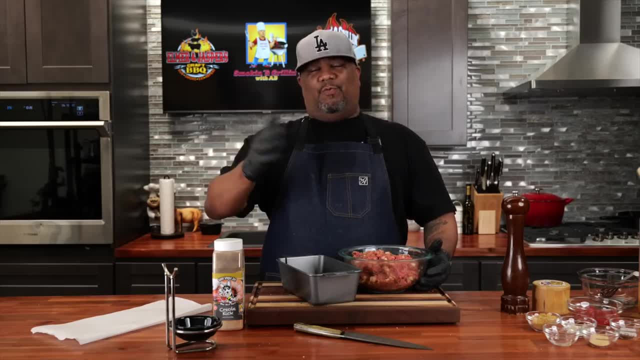 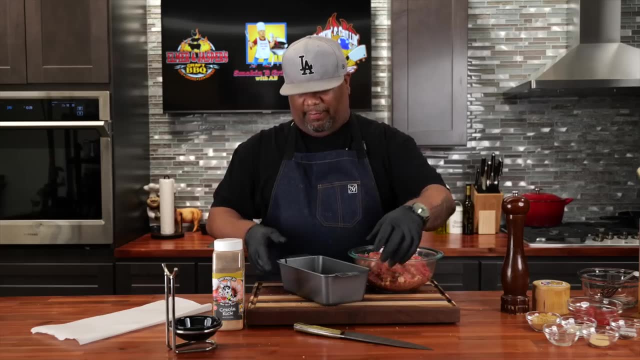 below. You know what it is and everybody gonna tell you it's the worstest. whatever it is, That's what it is. But you know, if you're watching this channel, we're gonna call it the W sauce. Now let me say, come on in here and I'm finna, show you how you get down right here, Okay, so look, now we're. 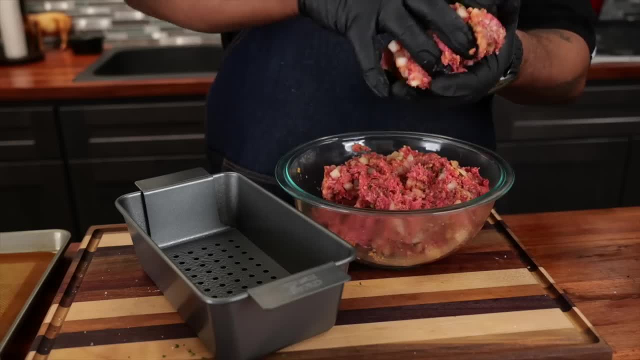 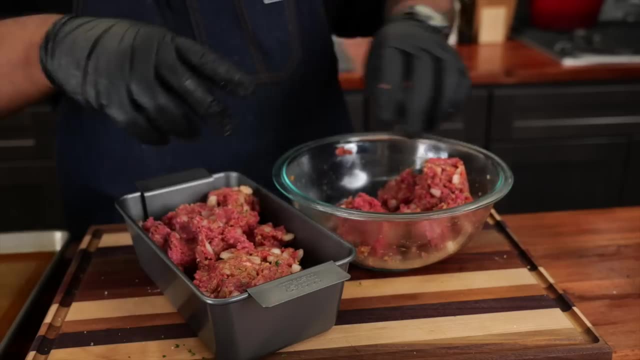 gonna go ahead and start filling up our meatloaf pan right. So for me, I just take it, and I don't want to push it all down right now. I'm gonna do it like this. Oh, you know what I wanted to say too while I was, uh, talking about things you can do to level it up. A lot of times, 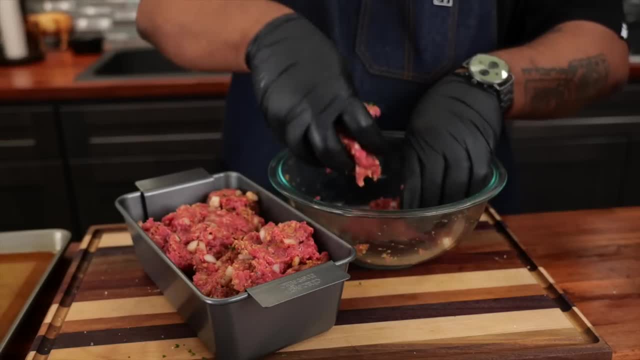 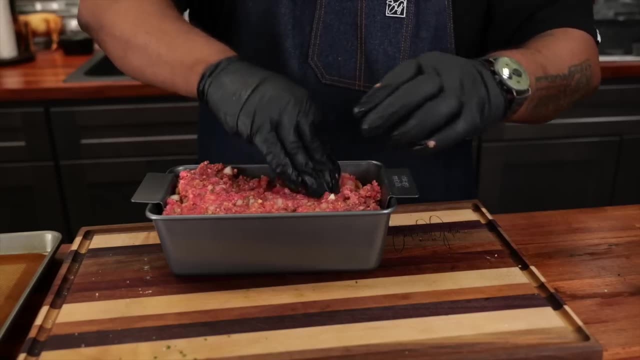 I use one pound of ground beef and I use a ground- uh- pork. You know what I mean. These are things that I do to make it, you know, super moist. Now, I'm not gonna pack this all the way down like you think, I'm just getting a sort of feel: Get rid of some of the air. 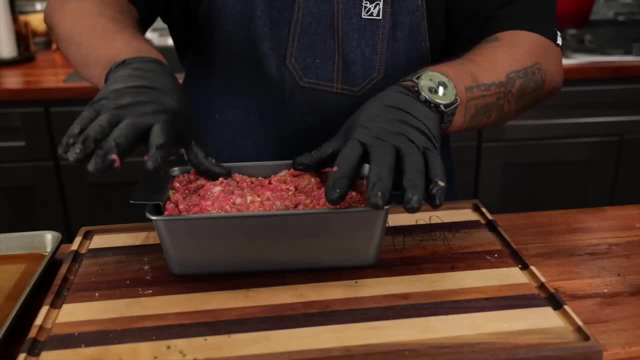 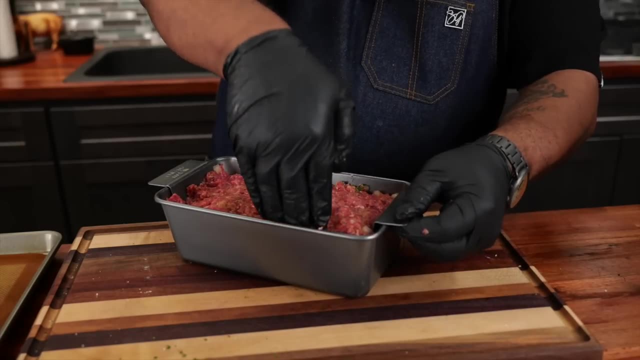 just around it, and then I make this little line. That's what I'm gonna show you, because you know what presentation is, everything right. Look, I'm gonna take my finger, I'll take these right here and I make a little indentation, as if I'm packing it down like that, Just on the edges only. 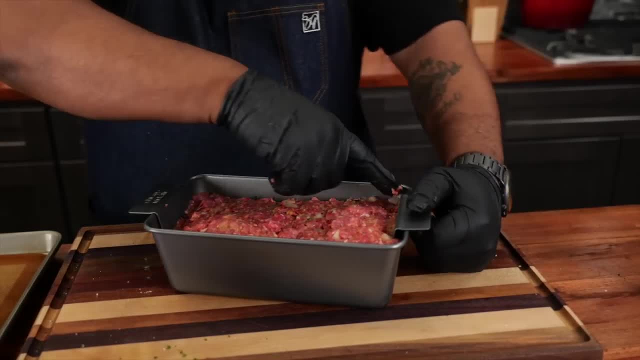 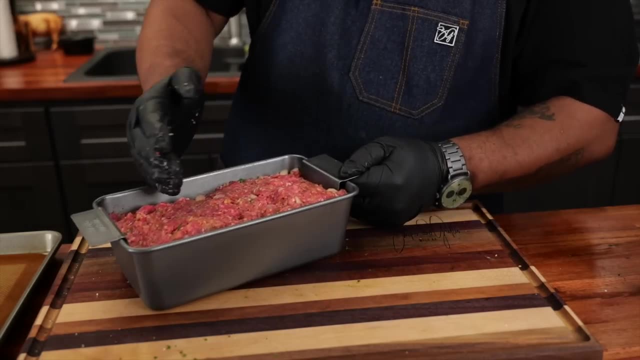 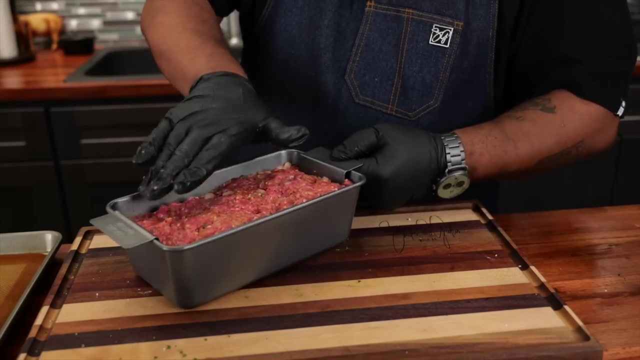 Then I take my finger, kind of like just bring it around and we're just gonna put an outline on it, just like this. So this part would be kind of like raised up and we go like that. Now I just want to get this pretty much level. Okay. so look, when you're done with it, it should look like that. 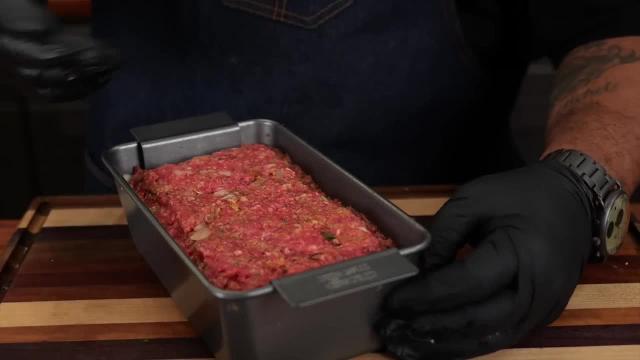 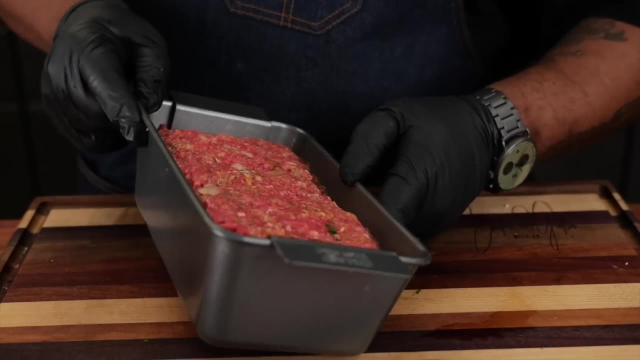 You can see, I made this little valley, this little edge right here, and my profession, what I used to be, that we call that a bevel, You know, I mean we just put that right there, It'll catch any of the fat that renders off on the side. Easy to get it off, all of that. and then, don't forget, we got it on. 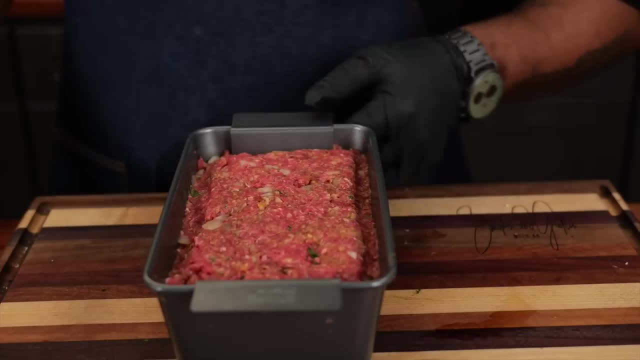 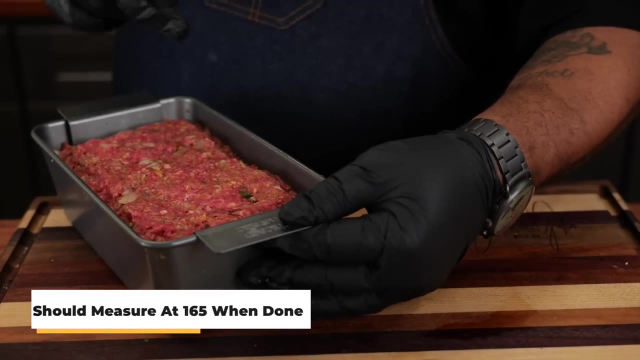 the bottom. Once it's cooked, we can lift it up. Hey, but enough talking. Look, I'm gonna put this in the oven for about 40 minutes. Well, how do we know it's done? We're gonna hit it with the meat thermometer, Stick it down in the middle and we're looking for 165 throughout. So we'll hit there. 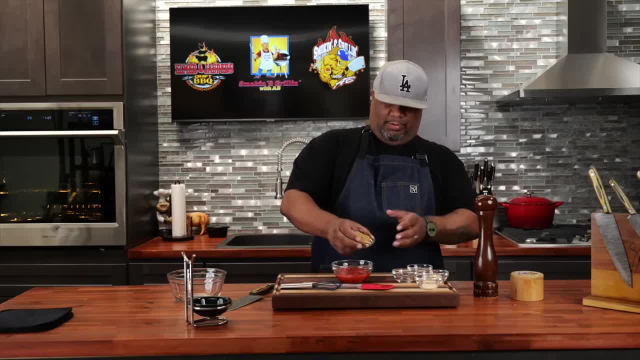 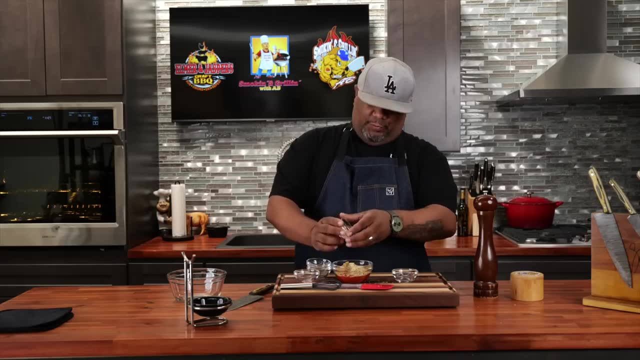 there and there. So we got our ketchup. We're gonna come with our brown sugar, salt and pepper. Hey, I want you guys to remember, listen. the whole full ingredient list with the measurements are down in the description box. Now get yourself a whisk. Those of you guys don't have that whisk. you know what we're gonna. 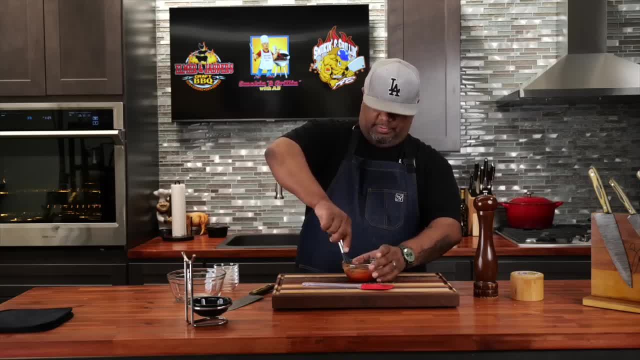 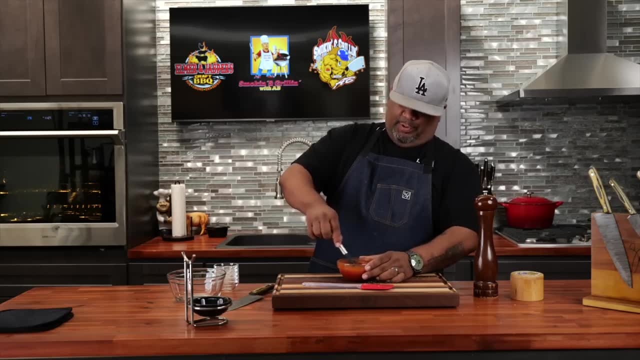 use. We're gonna go old school and keep it. you know, do it with that fork. Now that we got this incorporated, look most important thing. we got to taste as we go right. So let me go ahead and get myself a spoon. Hit it like this. This way we can make any. 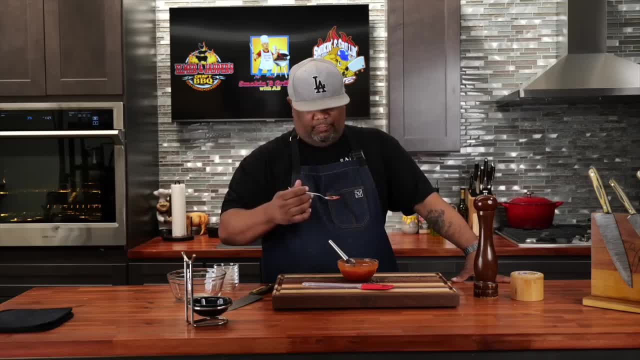 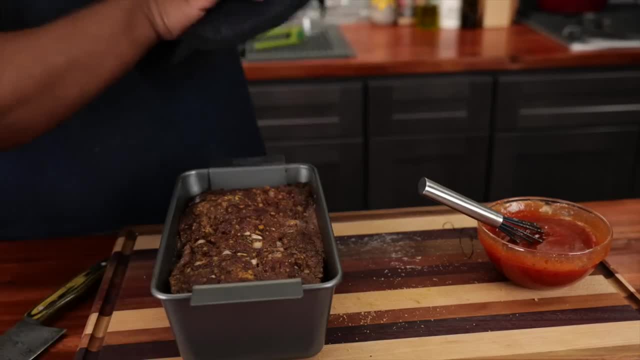 adjustment to it. right here, We got 1.45.. Don't need nothing, folks. Okay so look, my timer went off, Right? I just checked the internal temp. We're about 1.45.. But check this out, We're going to coat this. We're going to go back in the oven. 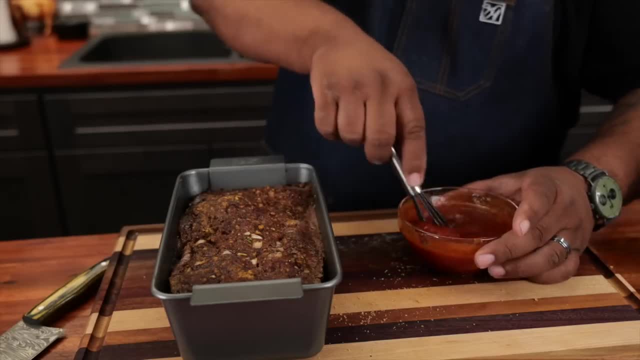 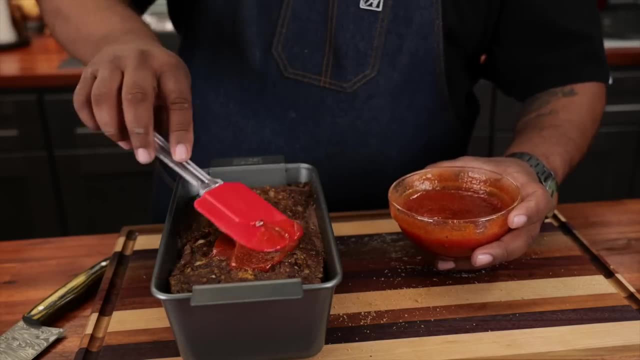 for about another 15 minutes, But what we're looking for is 165 degrees, And again we want it there, there and there. Now I'm just going to take this, and all we're going to do is just coat this on the top Right. 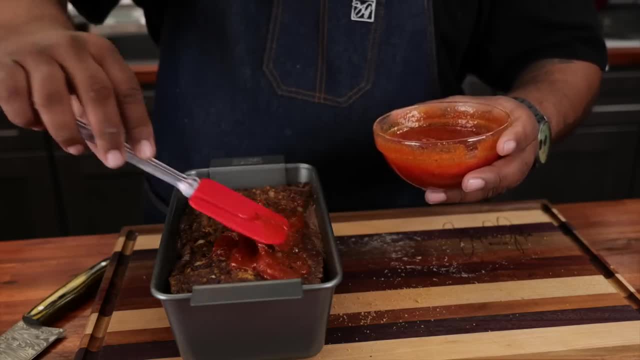 Then we're going to control it: 1.45., 1.45., 1.45., 1.45., 1.45., 1.45., 1.45.. continue to cook it now. there's a couple ways you can do this. you know what i mean, because we 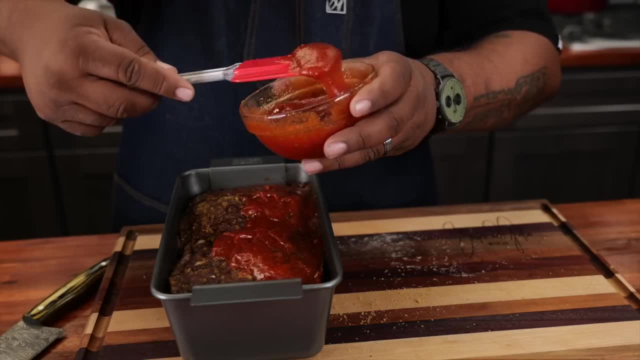 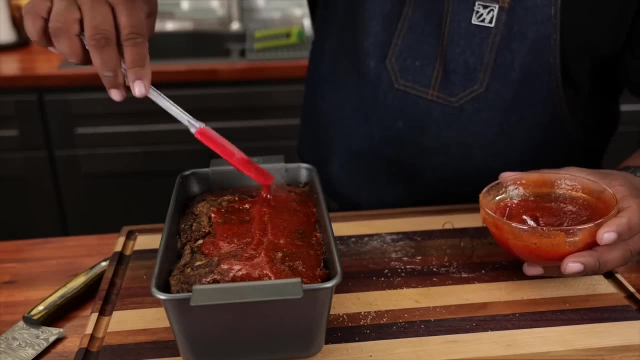 started out this way, just to get the loaf. i could have put this and put it on a pan right, that way we can get it on the side. hey look, we're not trying to over complicate this. this is going to be fire even when it's out and i get it set up, i'm gonna coat a little bit on. 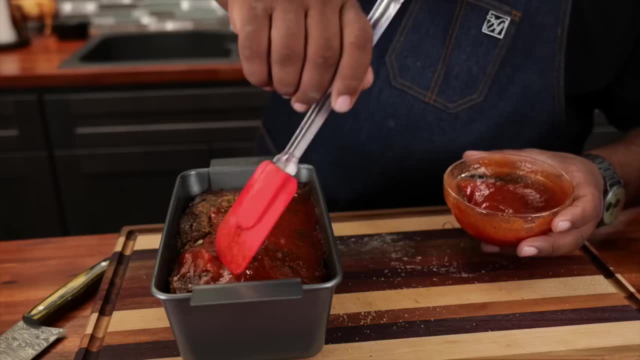 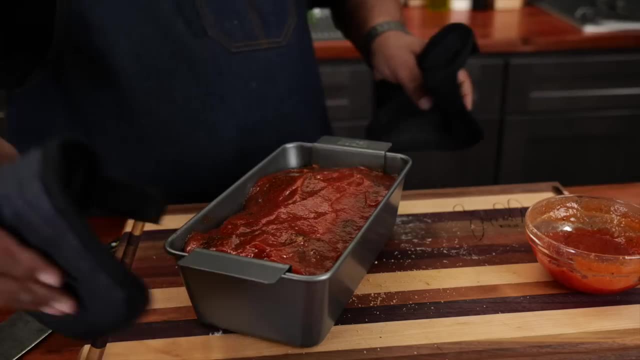 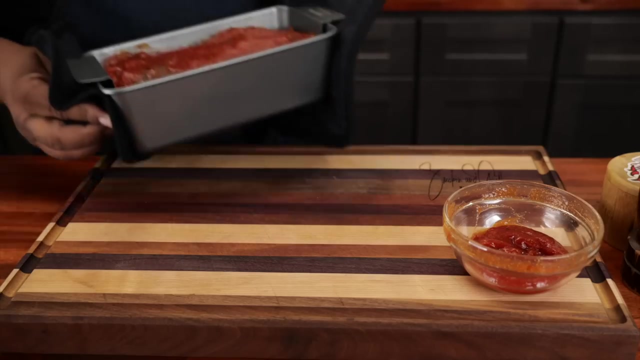 the side, anyway, you know, i mean it just won't be cooked on there like paste, but trust me, folks, it's still gonna be fire, okay. so look, now we're going back in, don't forget, we're looking for 165. we're gonna start our timer for 15 minutes, okay. so i want you to take a look at that right there. 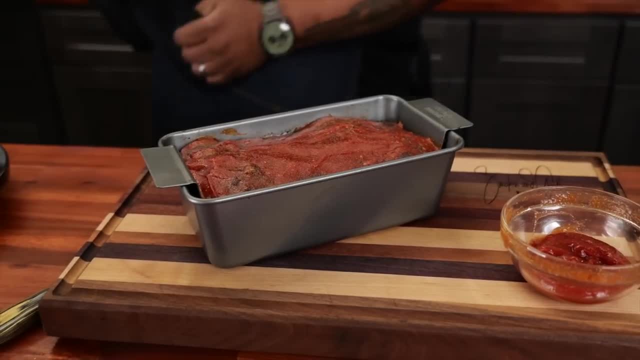 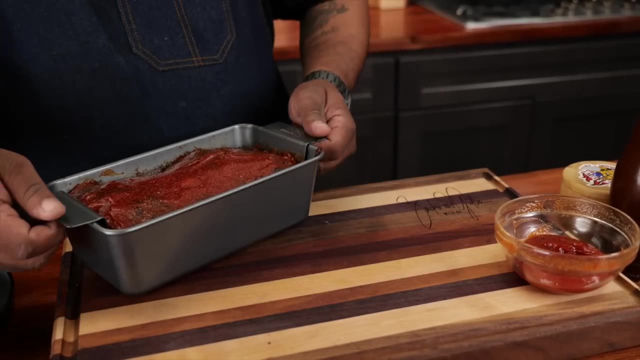 that right, there is just right. and i checked the eternal temp. we have 168, okay. so, look, i don't let it rest for about 10 minutes. actually it's been about 12 minutes, right, so i'm gonna go ahead and pull this up right now. you can see it just breaks loose. now i'm gonna run it like this just to get. 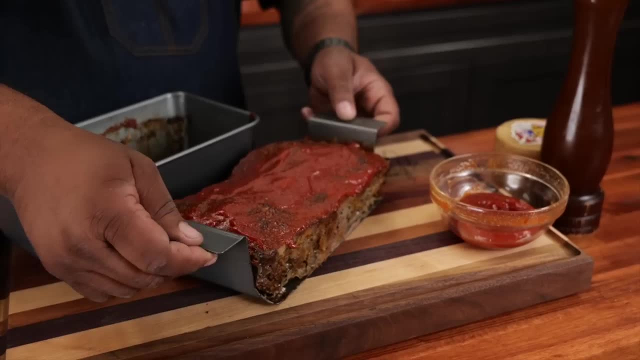 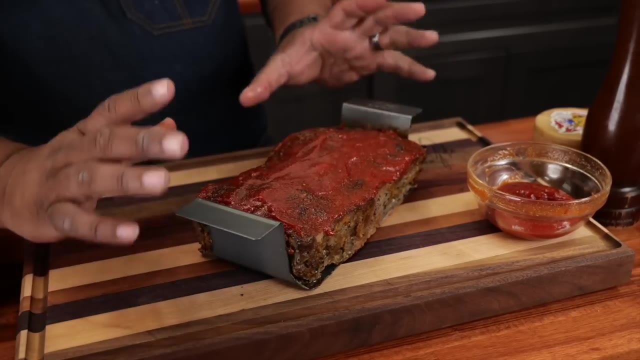 anything off the excess and i'm gonna just set it right here for right now. right and this: right here, we discard this. this is just all the fat and everything that came off. i'm gonna take my thumbs. look, if it's cool and you let it cool for at least 10 minutes, it should be be able, you know. 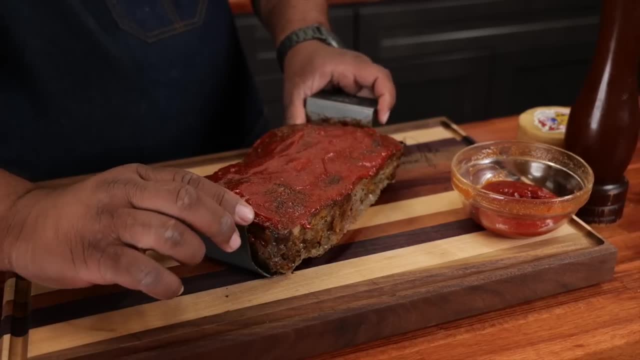 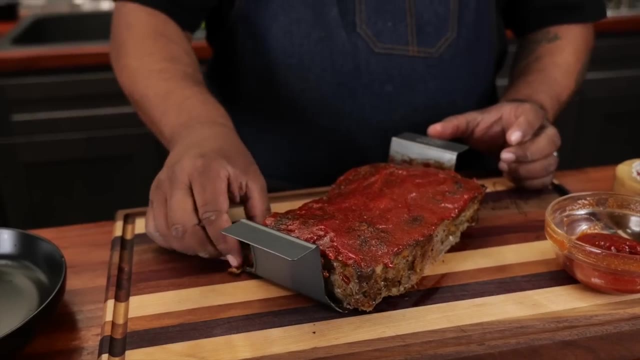 cool enough for you to touch it right, so i'm just gonna take it and you should be able to just slide it like this. we'll just slide it out. oh hey, check this out. this piece right here broke off. you know where it wrapped around this little part right here. but check this out, oh yeah. 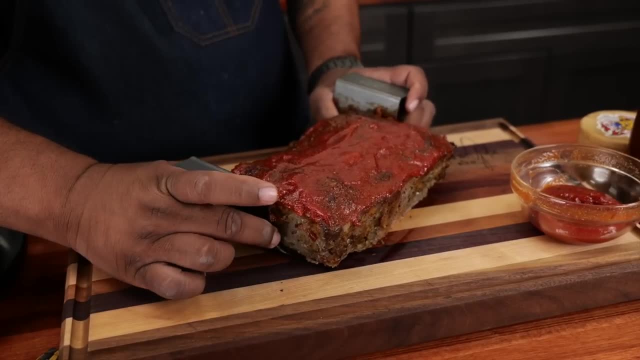 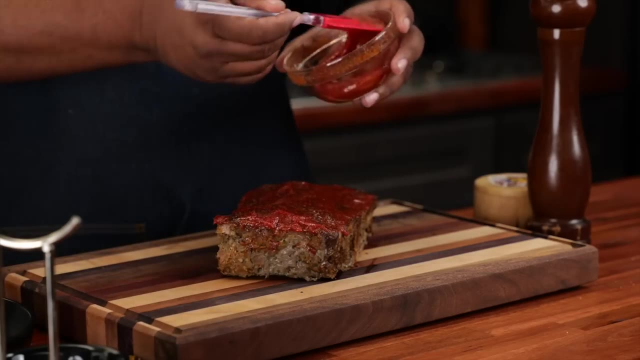 it's fire folks, all right, so we'll just slide this like this and let that rest continue to rest right there before i slice it. if you would like, remember, i'll save you some of this. you can go ahead and just put this on here like this: 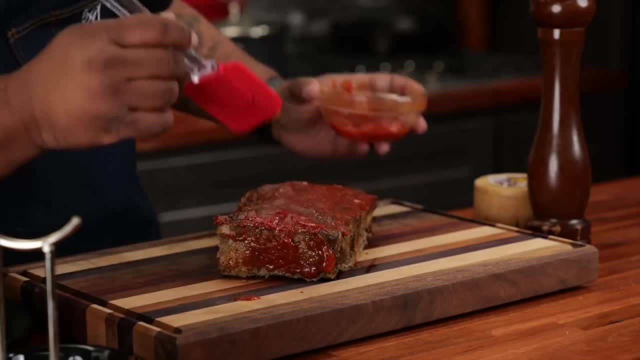 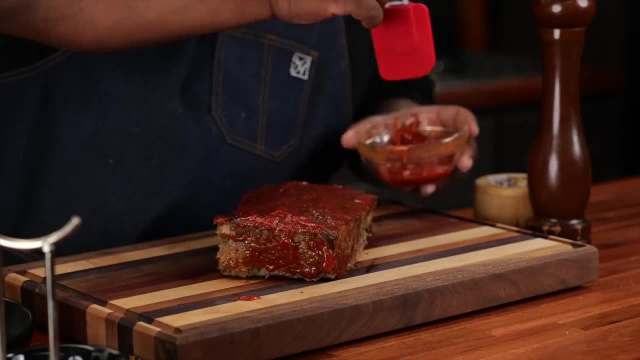 just to get a little coating, just to put a little bit more flavor on it. right, and don't trip. if you got one of my boards, listen, you've been cleaning it, keeping everything you know nice and clean. you know i mean it's sanitized, it's okay, you know. i mean that's why we got cutting boards. 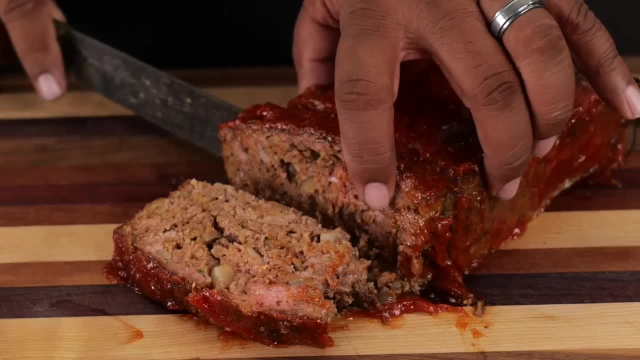 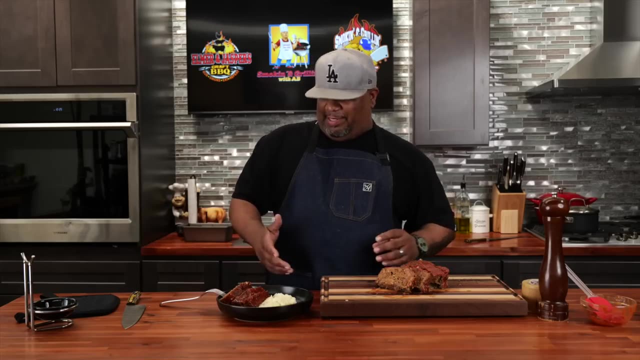 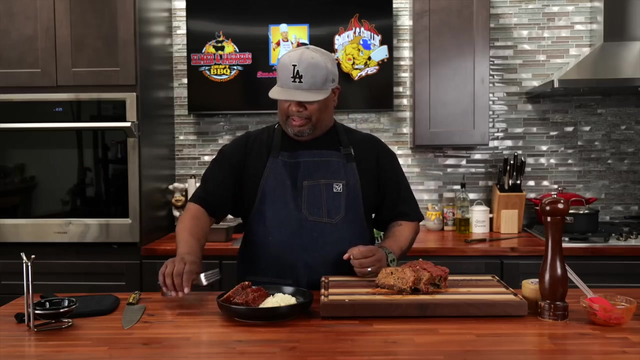 okay. so look, you can see me cut it. do all of that, and you know, of course you got to have the potatoes, right? only thing missing is, you know, the peas. you know if you want to keep it traditional, but listen, i'm gonna go ahead, cut me a piece, you know. i mean, hey, it's just super moist. notice, i don't use. no. 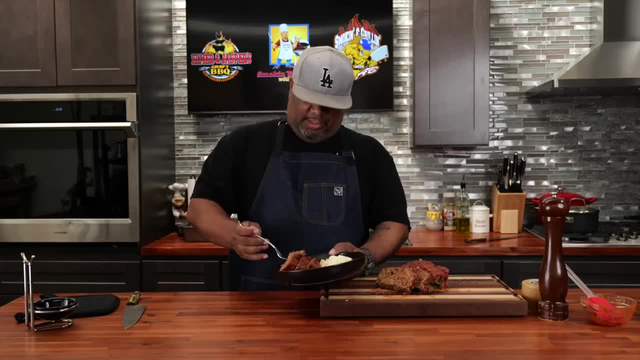 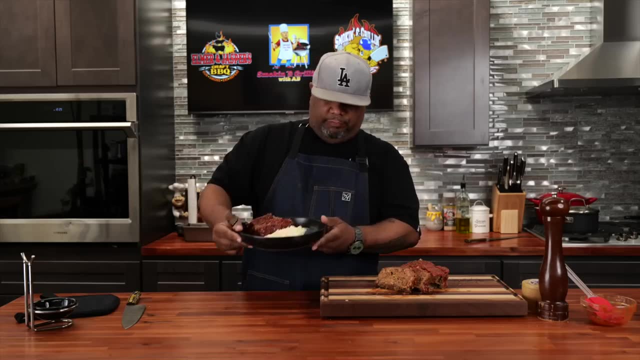 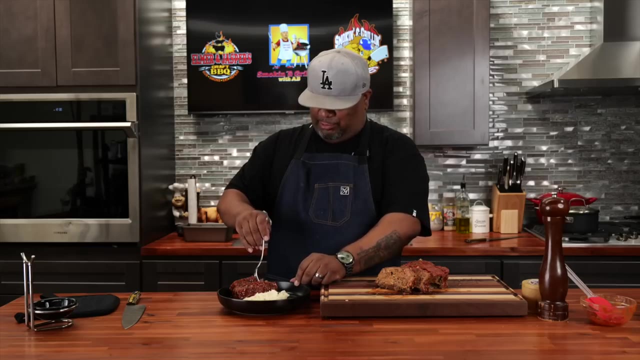 knife, you know, i mean we just hit it like this. this piece already broke off and ready for me. folks, cheers, i don't know i'm gonna go back, you know. i'm saying just to make sure i'm tasting what i'm tasting, right, oh? but i'm gonna go ahead and do it like this: get myself some of these mashed potatoes. 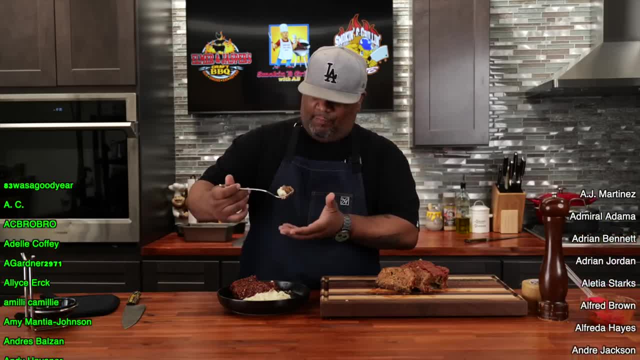 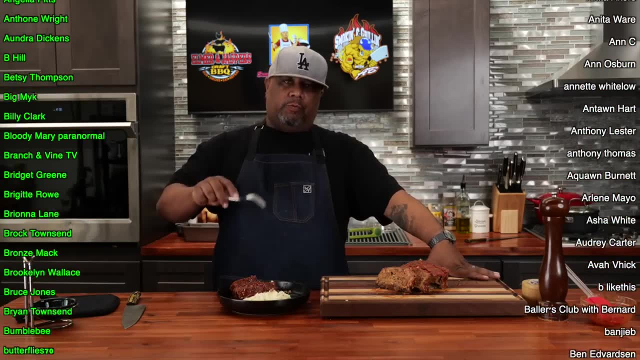 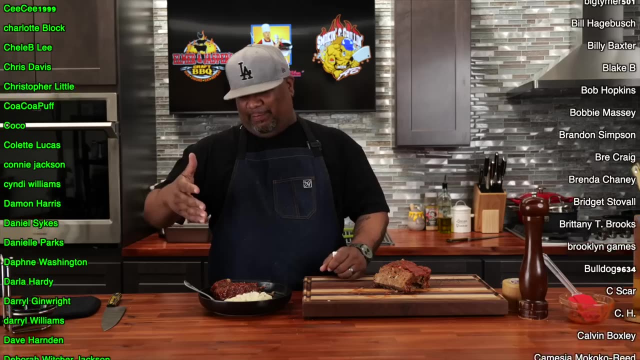 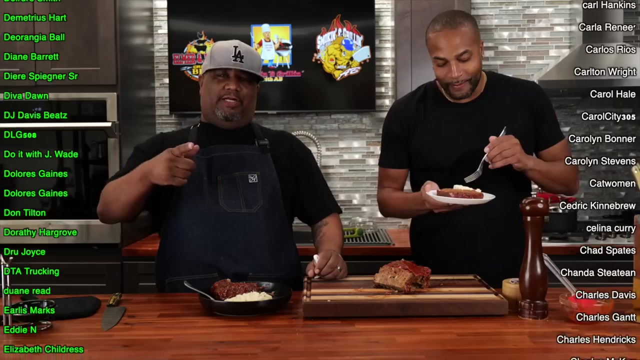 super moist meatloaf. hey, super fire, and i know all the time you guys get a chance to see me. you know i'm tasting the food and doing all that, but check it out, i got a guest. come on, man, bring yours over here. look, you guys should know him. you know he was in the last podcast. hey, i'm gonna introduce him how he